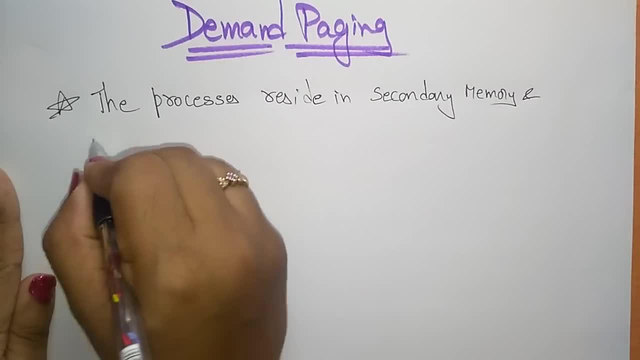 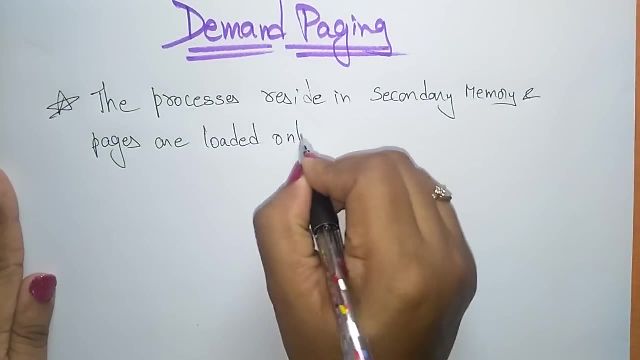 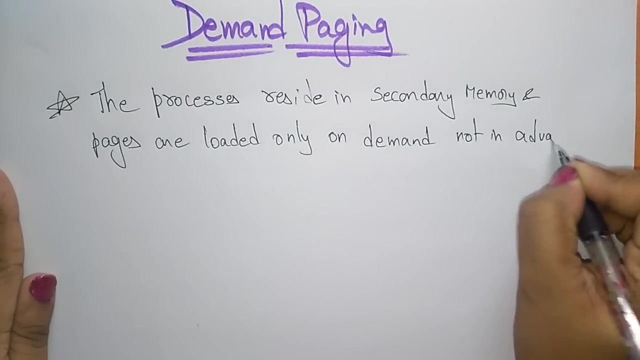 resides in the sec secondary memory and pages are loaded. and pages are loaded only on demand, only on demand, not in advance. so actually, the main memory starting whenever you switch on the computer, the main memory, that is, everything will be free- means that the main memory is nothing but a ram. okay, random access memory. whenever your system is on, the ram is free. 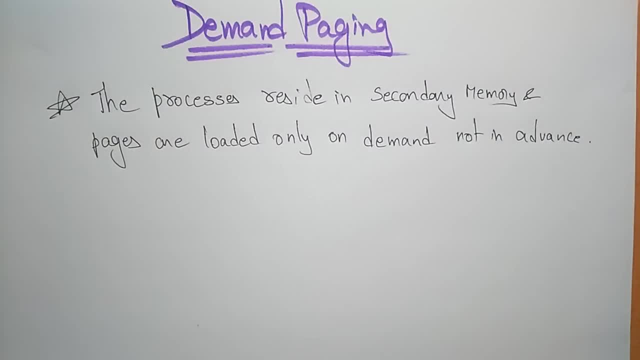 so it's free. so whenever the process, uh, everything the process, are present in the same condition as the very first one and the other one that are being opened, if the second memory so, and the pages are loaded to the main memory only in on demand, not in advance. so 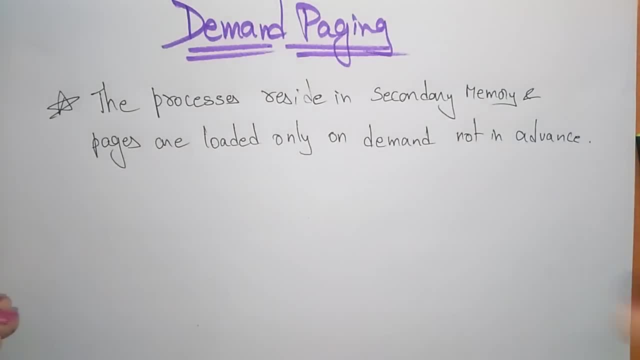 whatever the page you are opening means whatever the folder you are opening. so that is present in the secondary memory, so it will be. everything will be stored in the main memory. so it will be. everything will be, uh, stored on the basis of demand, not in advance so that you call conclusion. 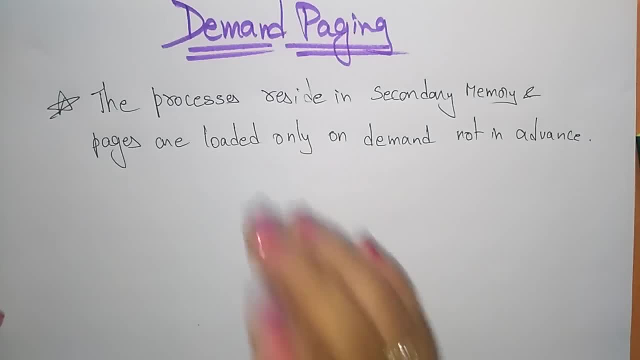 it as demand paging so by the processor. the cpu wants to execute, suppose, if it wants to retrieve a file from the secondary memory. so uh, first, whenever that it goes to the secondary memory and uh, bring that page or a frame to the main memory. let me explain with an example there. so let us take this is the main memory. 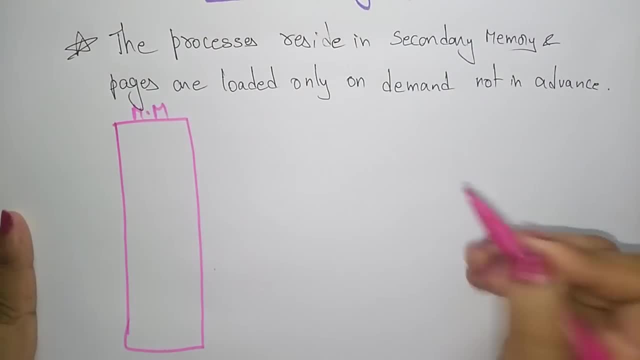 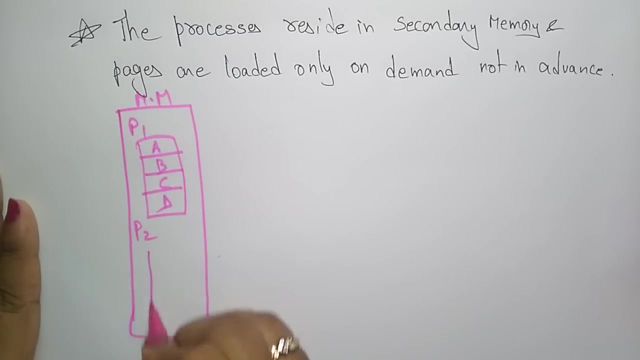 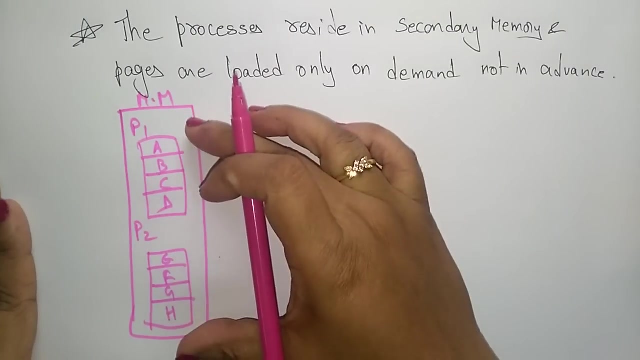 so main memory consisting of process p1 and the p2, two pro. sorry so each process having some frames- a, b, c, d, like that- and the process 2 is having e, f, g, h. so the main memory is having already it is full, it is having the frames and coming to the secondary memory, 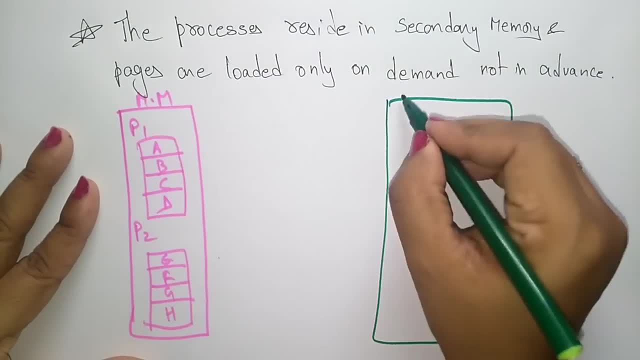 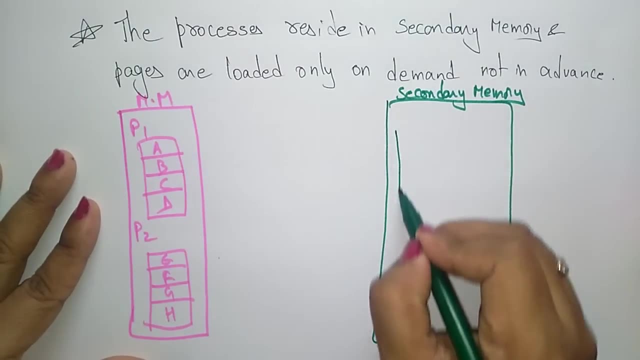 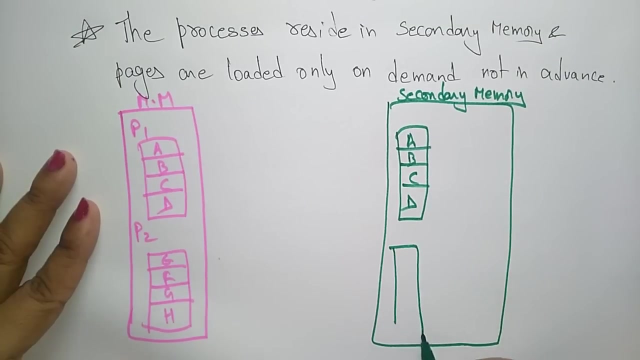 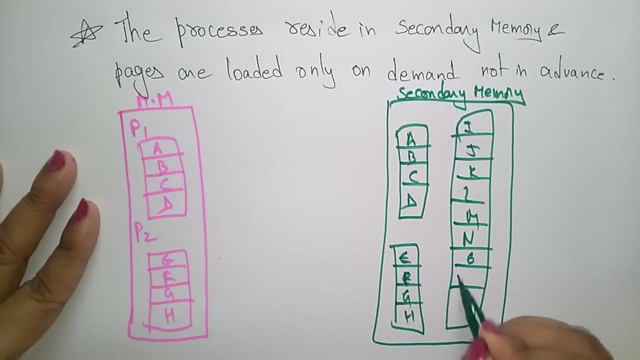 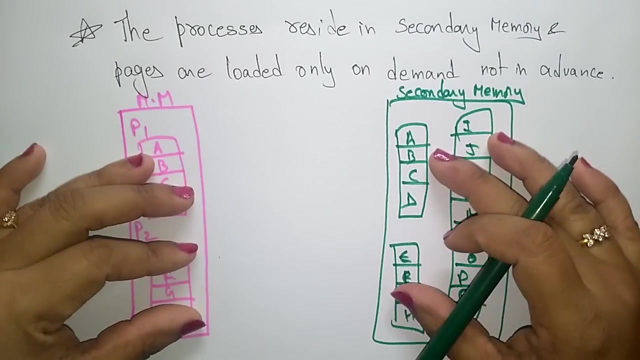 secondary memory is the disk. this is the secondary memory, so the secondary memory consisting of, suppose, a, b, c, d, e, f, g, h, i, j, k, l, m, i, j, k, l, m, o, please, p, q, p q. okay, so this is the uh pages that are present in secondary memory and the main memory. 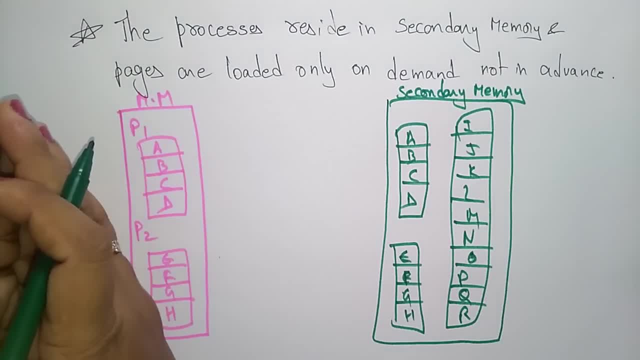 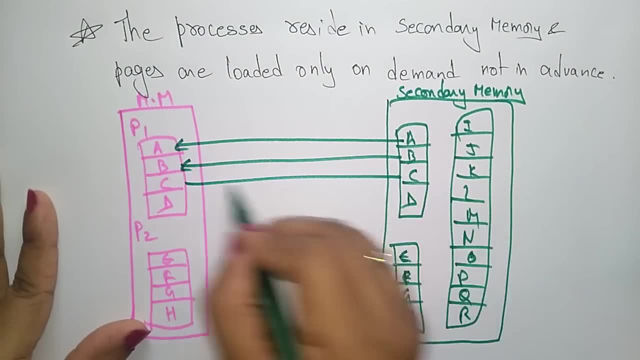 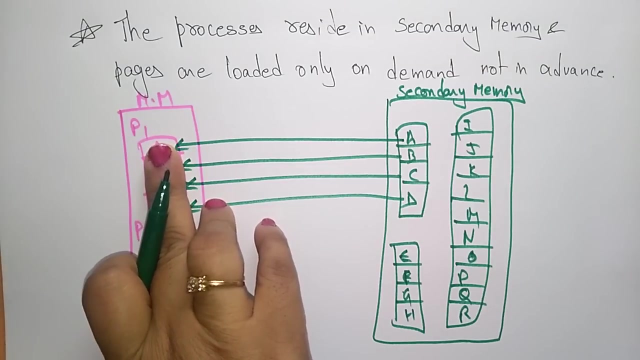 so whenever the processor is demanding for process p1, that data will be stored in main memory. so star it starting. all the frames are free, the data that is. uh, the main memory is free. so whenever the cpu demands, cpu demands free fantasy or lavalier network. 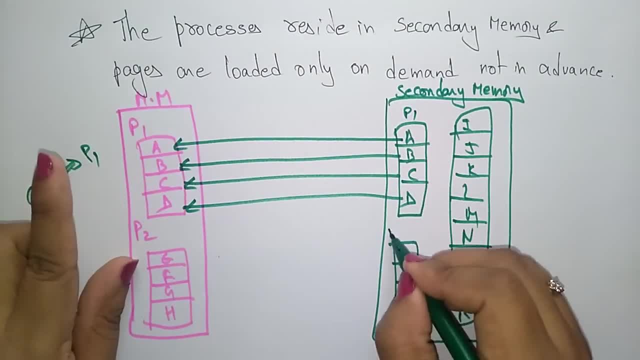 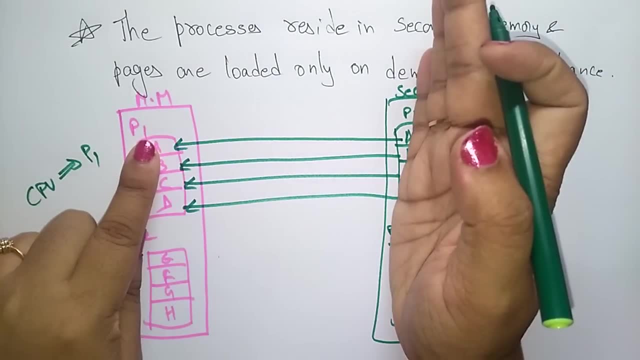 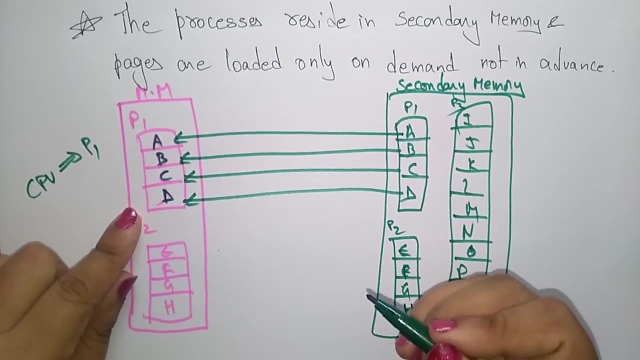 for process 1, p1. so this is the p1, this is p2. let's take this is the p3, like that. so whenever the process cpu demands for p1, so the data that is present in the secondary memory will stored in main memory. a, b, c, d- okay, suppose, if you want to store these data, some data in the process p2. 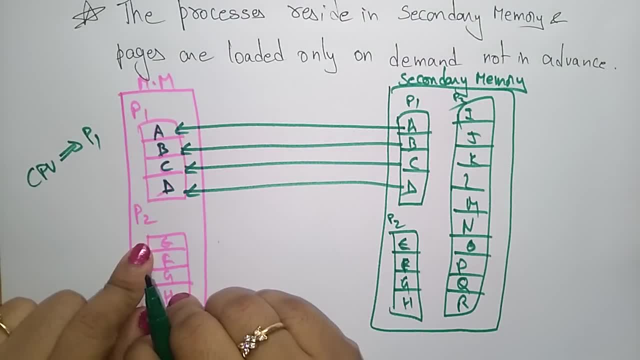 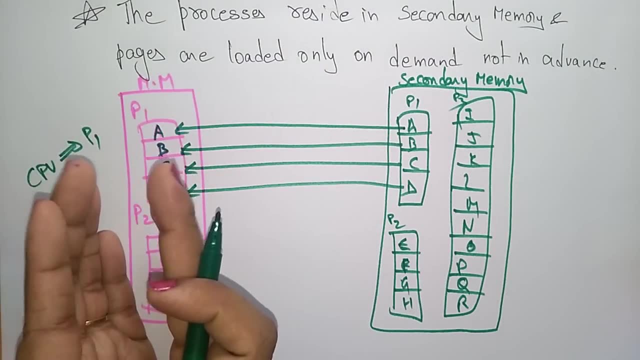 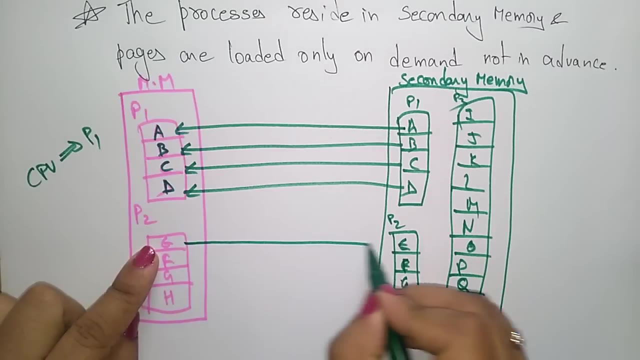 but here it is already full. the process p2 is already load in the main memory. if there is no space in the main memory, you just if. if you are not using process p2, okay, you just send the data to the secondary memory and takes the new data, okay. so now i want to swap out this: 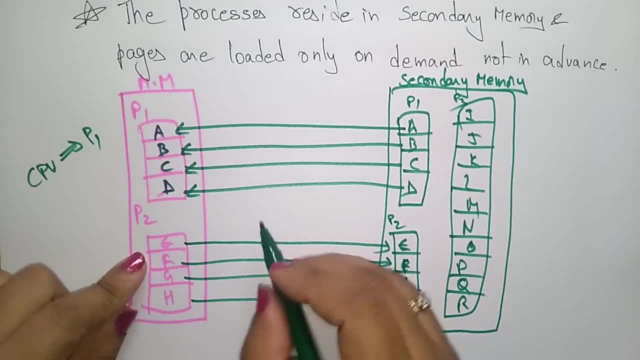 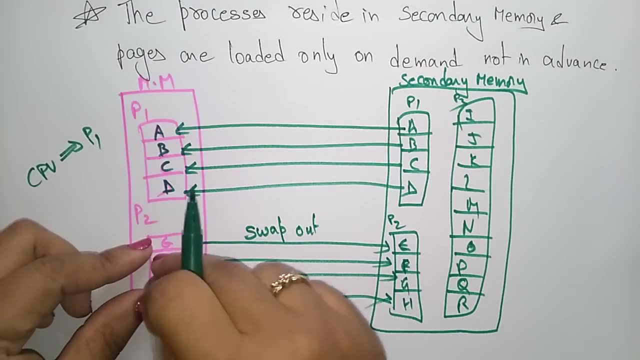 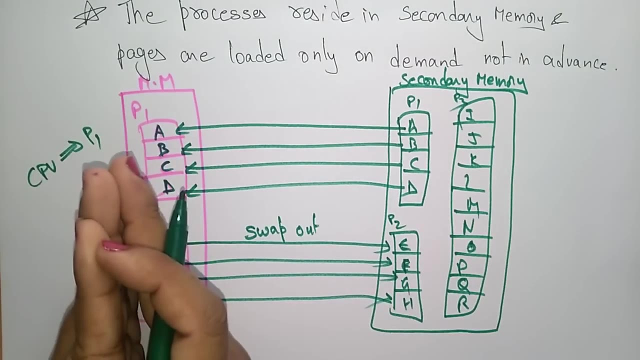 process. so this is the swap out. so whenever there is no use of pages in the main memory, if you are not using those frames in the main memory, you just again send that data to the secondary memory and take the new data. so whenever this operation is over in the main memory you can again swap in. 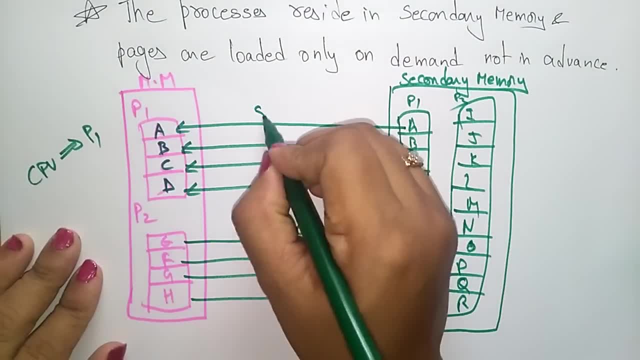 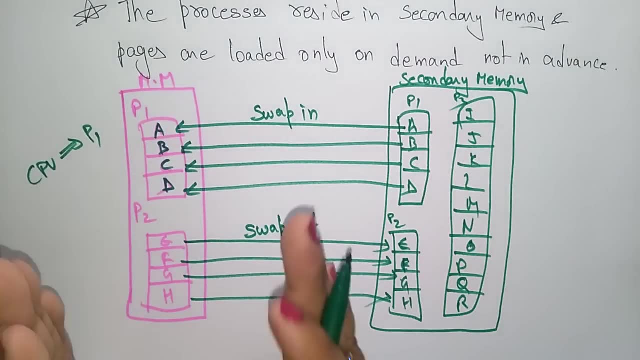 the already swapped out data. so this is a swap out and this is a technique of swapping. so it is just similar to the paging system with swapping. so the demand paging is everything is depends upon the swapping. so you have to demand the page from secondary memory. the cpu is demanding the page. 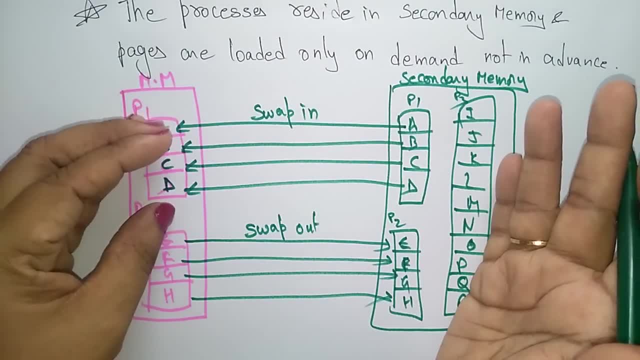 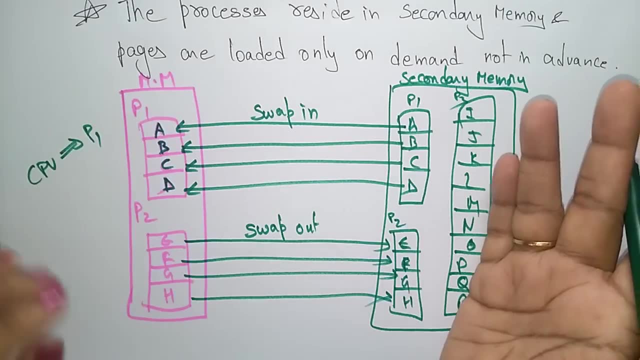 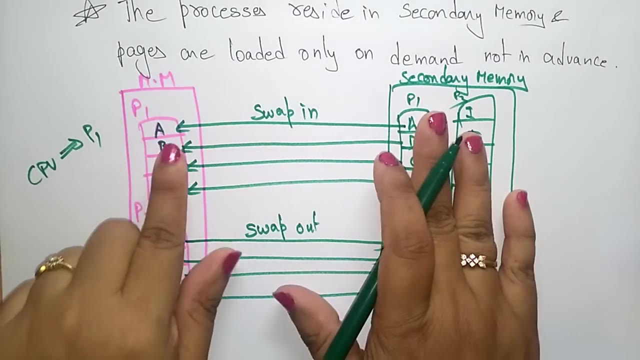 from secondary memory. suppose, when the main memory is not free, you just swap out the page that are not used in the main memory and place the new pages in the main memory. so when we want to execute a process, just swapping if you want to execute the process, just swapping if your execution 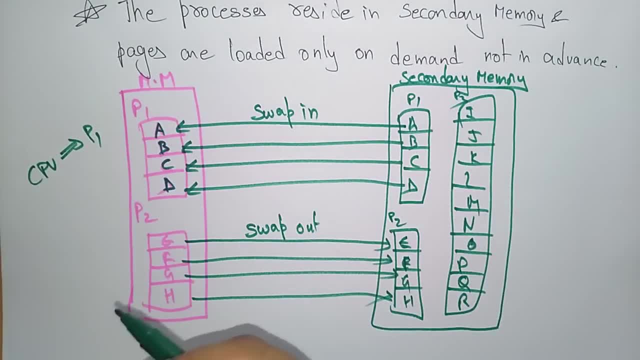 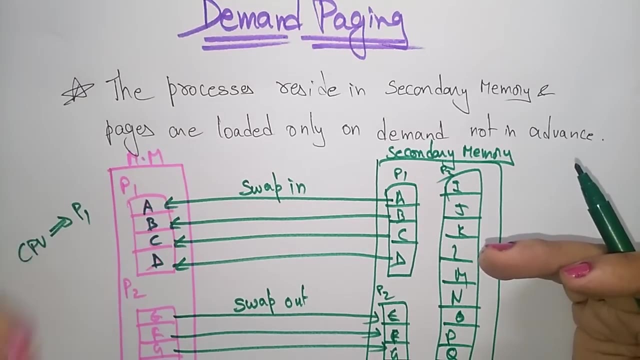 is over, just swap out. don't bring the pages in advance. so the process resides in secondary memory and pages are loaded only on demand, not in advance. so that is a concept of demand paging. so while executing that, if the program refers pages, okay, while executing the program, if the program refers. 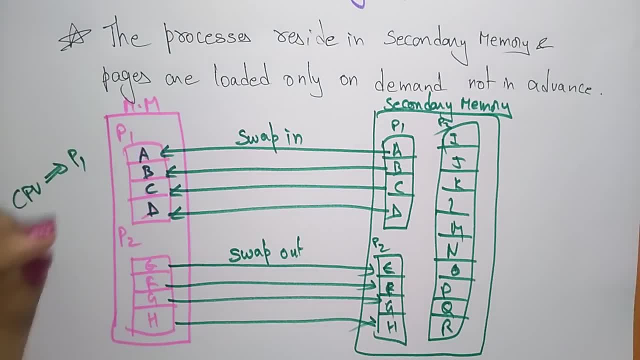 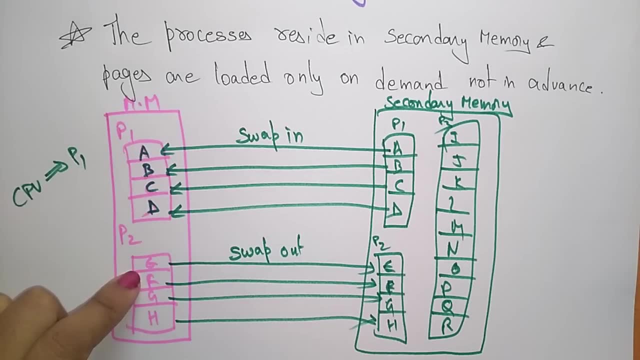 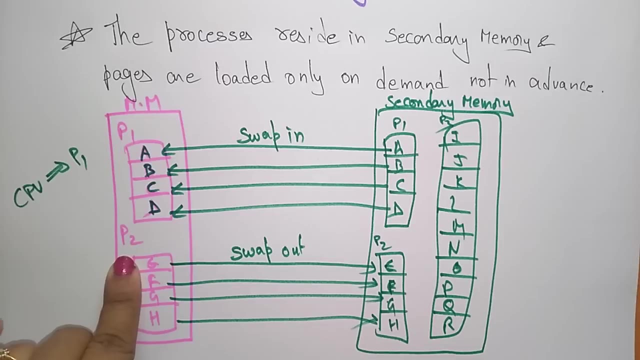 pages which is not available in main memory. suppose if, if i want some page, so that page. suppose i want the e page so, which is not available in main memory because it was swapped out little ago. so i just swapped out, but i it is not present in the main memory. but cpu is asking. 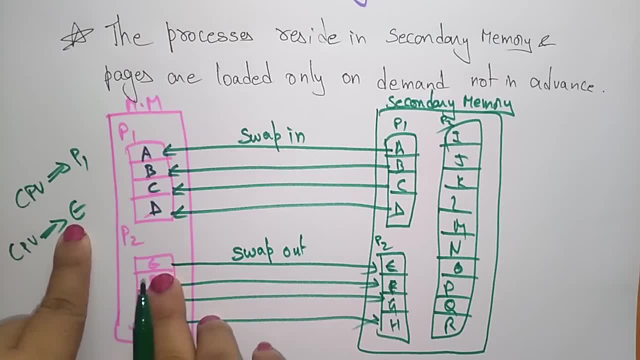 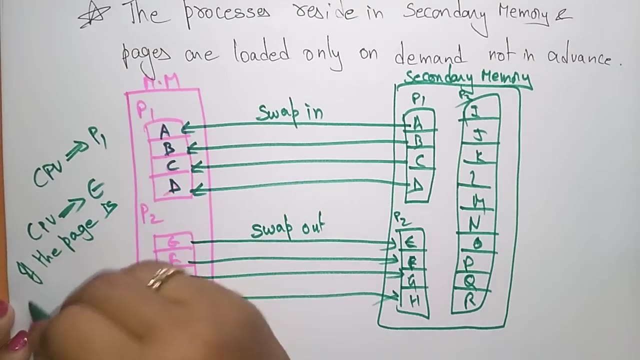 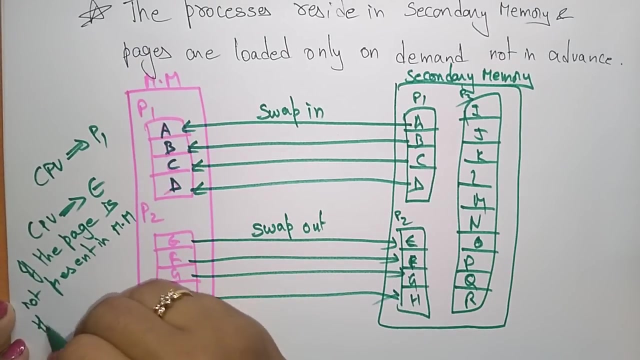 for e page. CPU is asking for e-page but it is already swapped out, then the processor treat this invalid reference as a page fault. So if the page is not present, page is not present in main memory, then we call it as page fault. 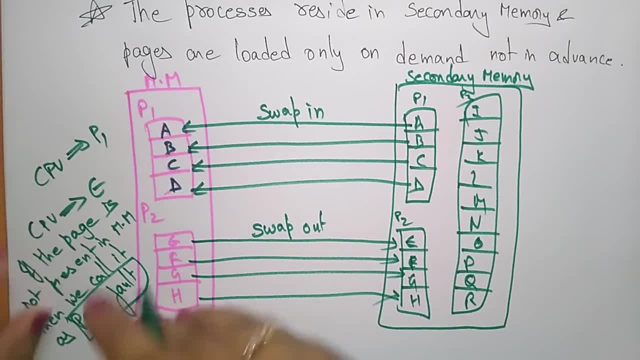 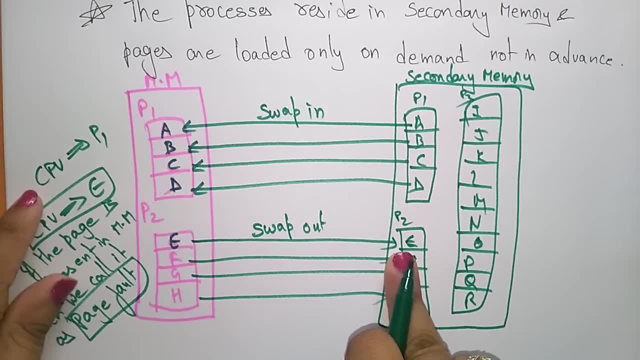 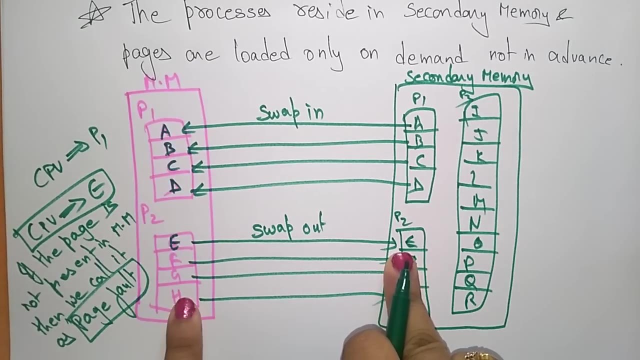 When the demanded page, the CPU demands the e-page, but e-page already swapped out to the main memory. but CPU is asking for e-page. So if the demanded page is not present in the main memory, then we call it as a page fault. 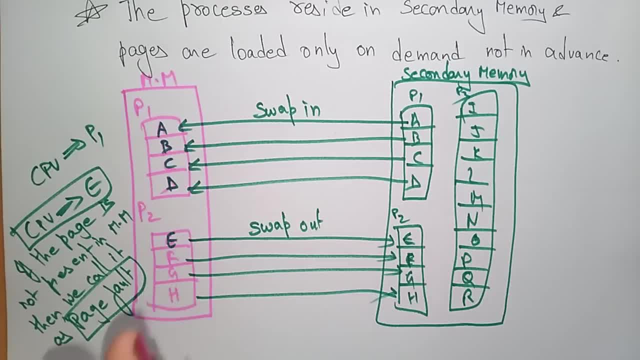 OK, So what does the processor will do If the page fault is occurred? okay, the CPU wants ePage, but that ePage is not present in the main memory. then the CPU transfers a control from program to operating systems to demand the page back into memory. 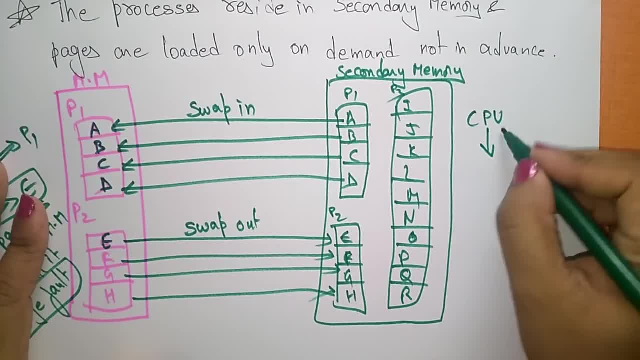 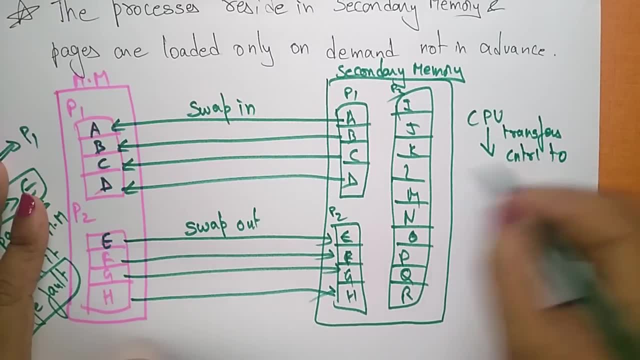 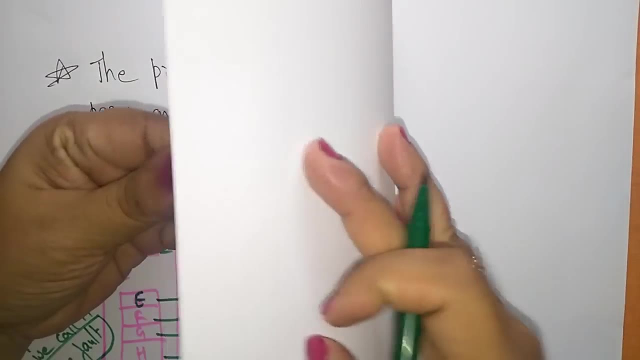 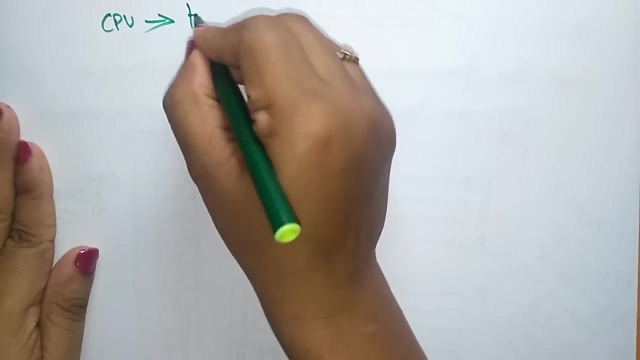 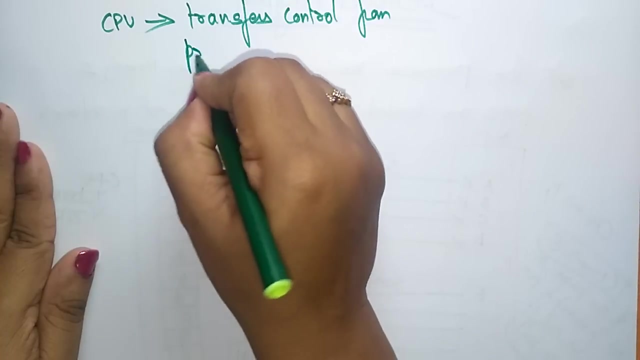 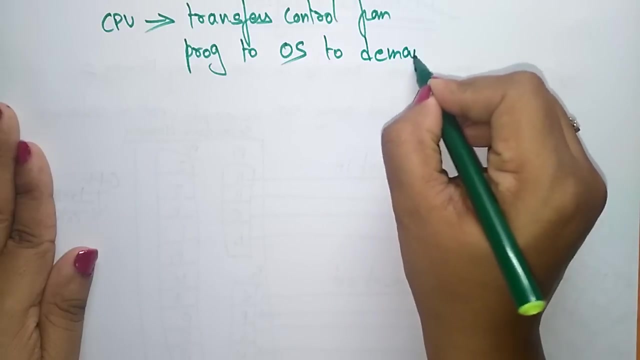 So CPU: CPU transfers control to control to control, transfers control from the program to operating system. So not like that. let me write that. So if the page fault occurs, CPU transfers control, transfers control from program to operating system to demand the page back into main memory. 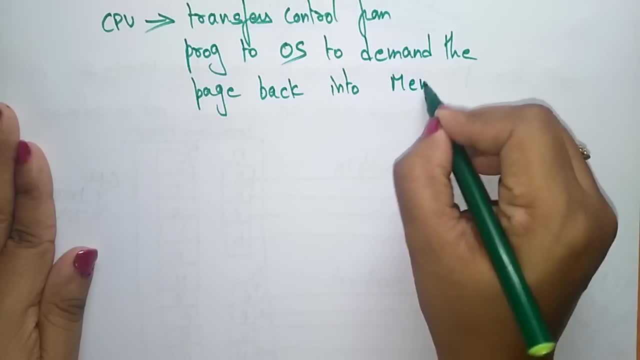 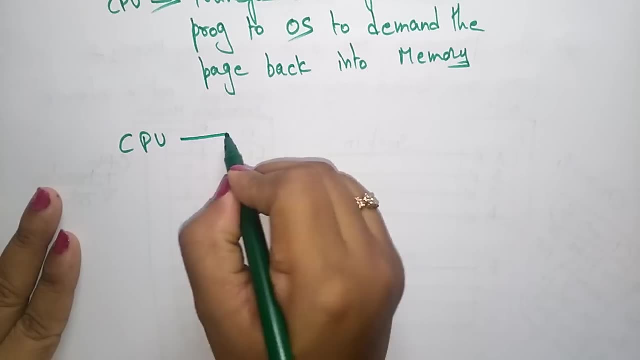 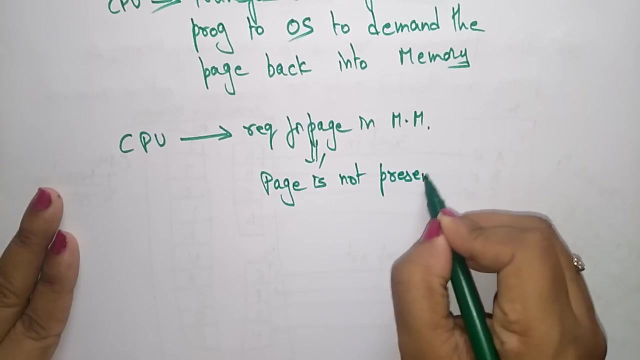 Okay, So that is the concept. okay, Suppose the CPU is requesting for page page in main memory. okay, Suppose the page is not present. page is not present, So whatever, the requested page in the main memory that is not present.